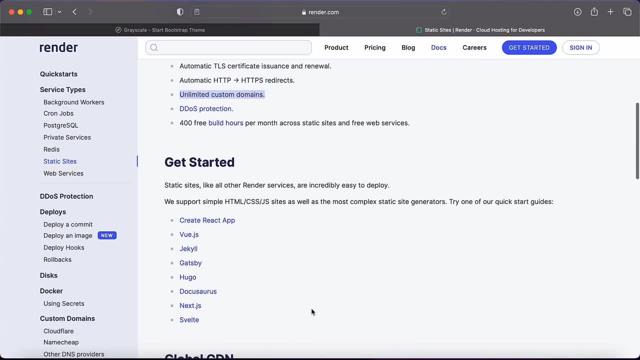 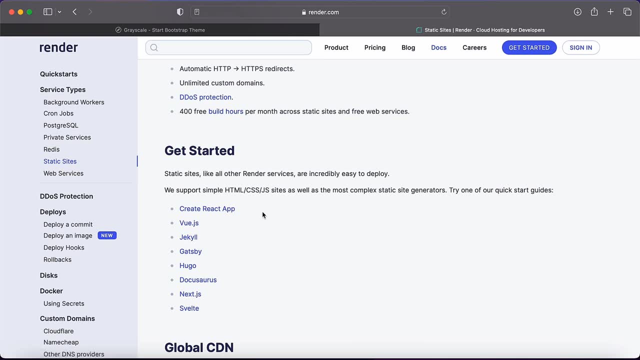 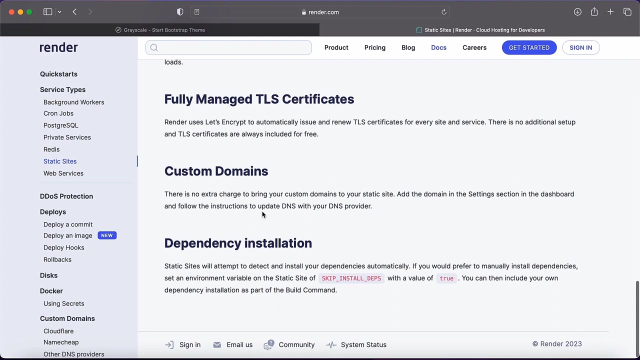 their own custom domain, but here they allow us to use their custom domain, our custom domains, and here list of the type of static inside. you can try even you can rear view kind of static content you can try so you can check in. here I'm only use simple HTML CSS one. yeah, here you can see you can use the custom. 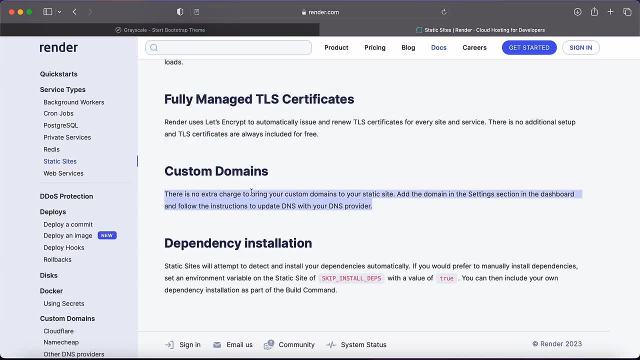 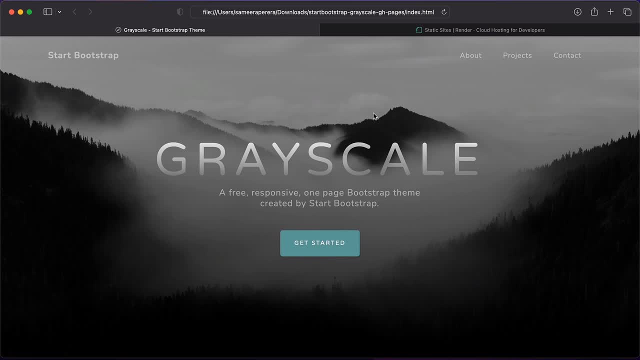 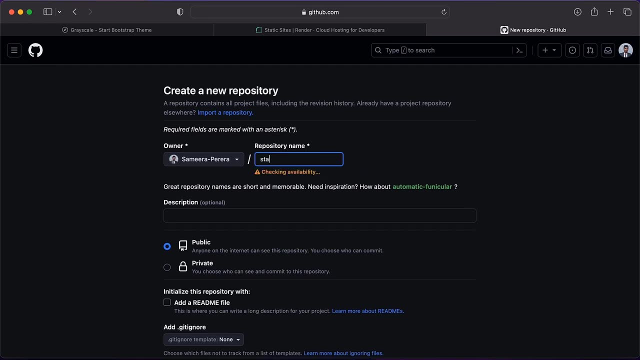 domain. so this is our website and let's start with creating new github report. so hope you are already familiar with github. if you're not, please comment below. I will do another video for the explaining github. so in here I'm creating my own repository, just simple repository, and yeah, keep it as a private, because this is your private. 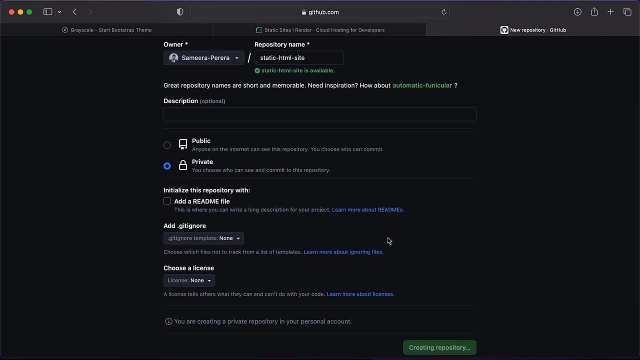 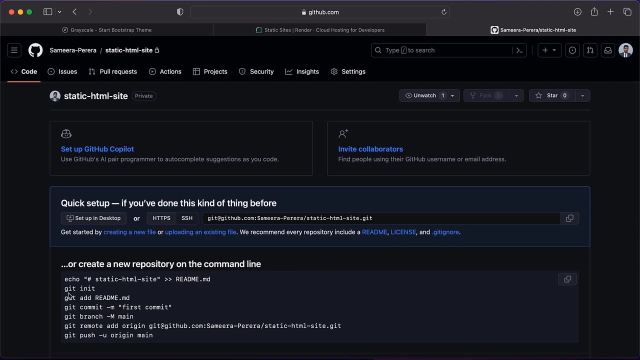 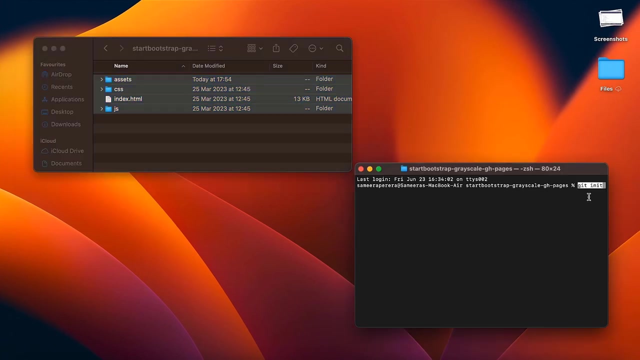 code, source code is keeping private. and yeah, just then you how to simply create github project files, your source code. so I'm following this command. so I already hope. on the command line, my project folder, I simply adding this command function for my project folder and厞 Slain's well, I put here key and expanding the Japanese. 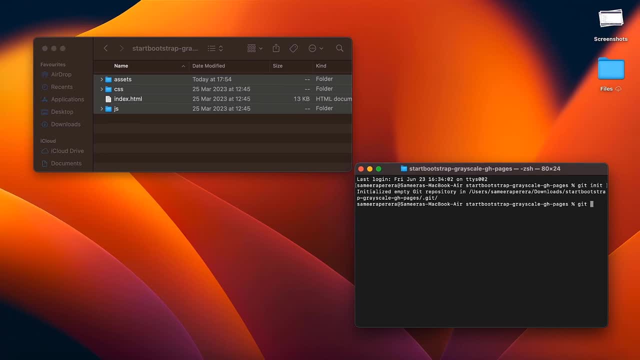 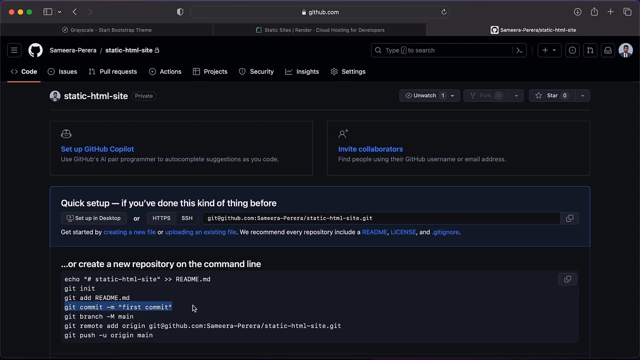 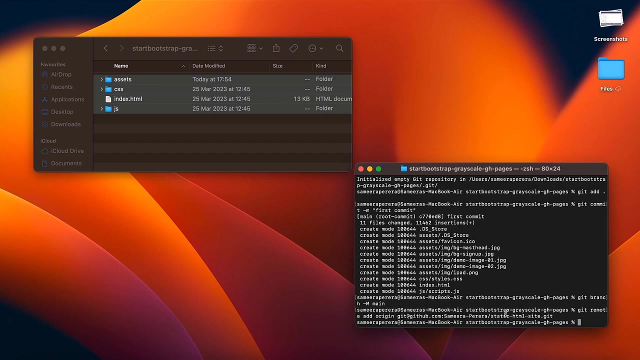 chit, add, call, commit the change my bus, commit and create main branch and add the remote repository in here i am using ssh, so if you are using http you have to check those. so if you don't familiar with github, please comment below. i will do another tutorial for that. so and finally, yeah. 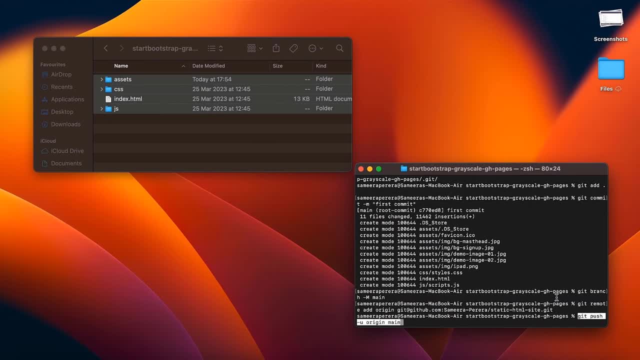 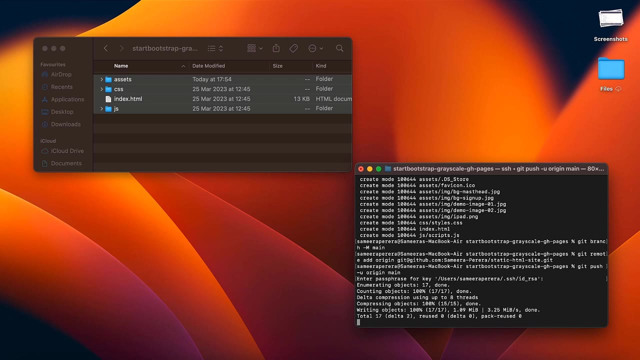 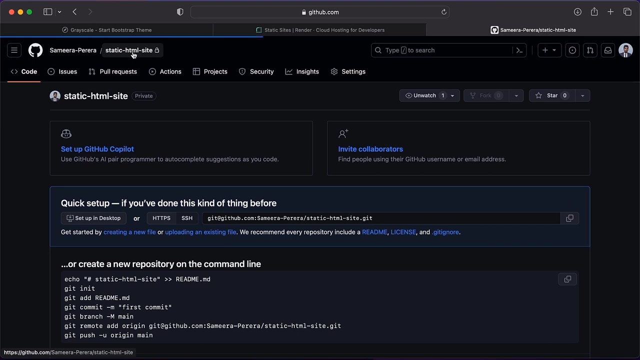 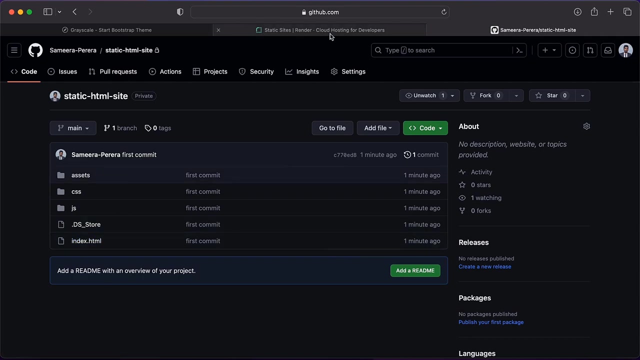 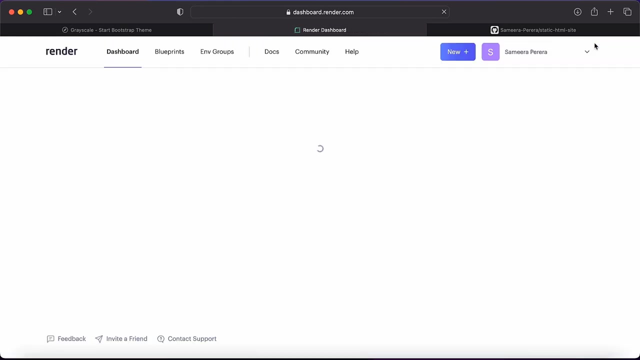 pushing, i make my password and it's done. let's check our website. let's see: okay, our old file. now push into you github. so then you have to sign in render hosting site. i'm just using my google account. i already signed in, so just so you can see. 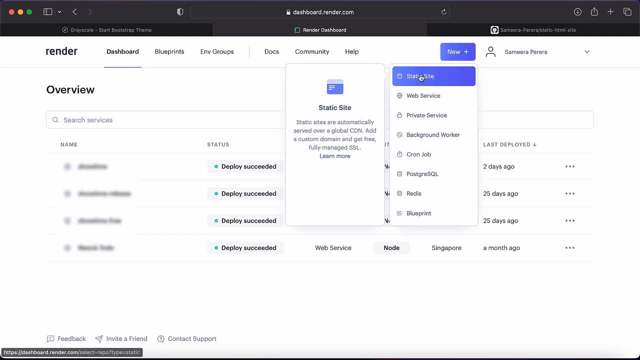 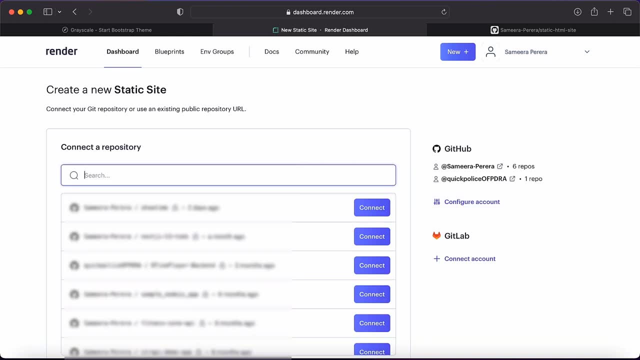 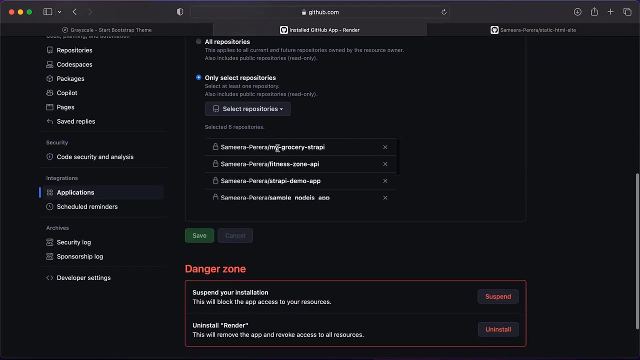 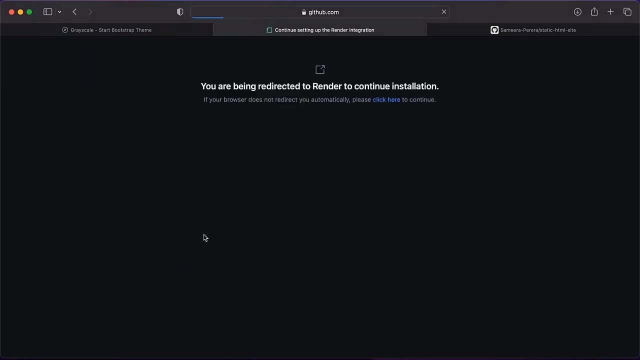 here i have several project already created. i will create static site from here and in here. if you are already connected to your github account, it will load your repositories. i will, but i am not giving all the repository access in here. i will manually giving my repository access. so i will select repository and save. now it will redirect. so 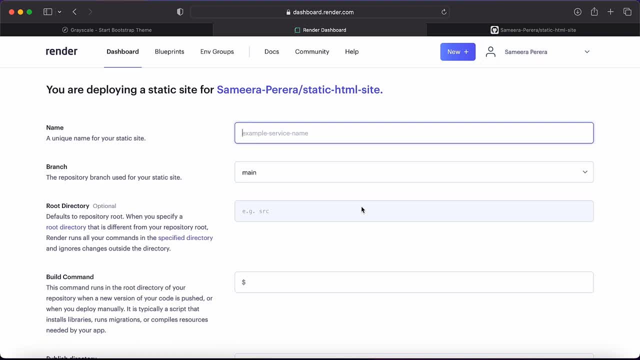 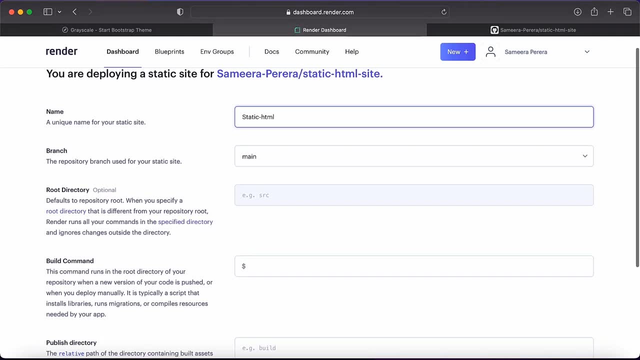 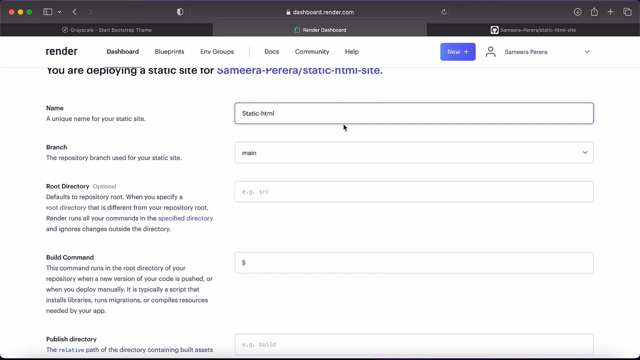 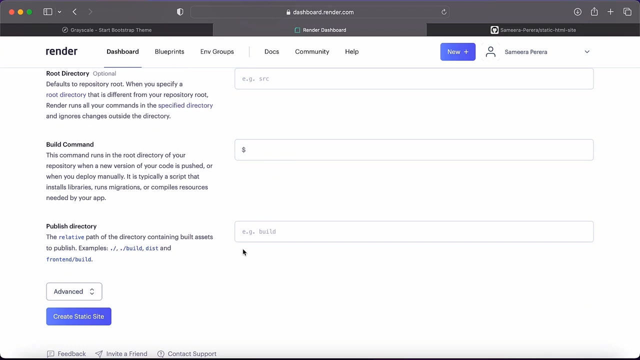 you can see here, see your repository, then click connect and here you can give some you want and you don't have much configuration to do in a static website. in here you can select your branch. if you have a different branch for production, i will keep it is in main and i don't. have bil command and in advance, so names would be pretty much the same. scaling administration right along for the next page in views is like that: go from here and go to settings and go to my backend button. us fees will be the same as on web site and i hide it in my mind. if you have options, you can. 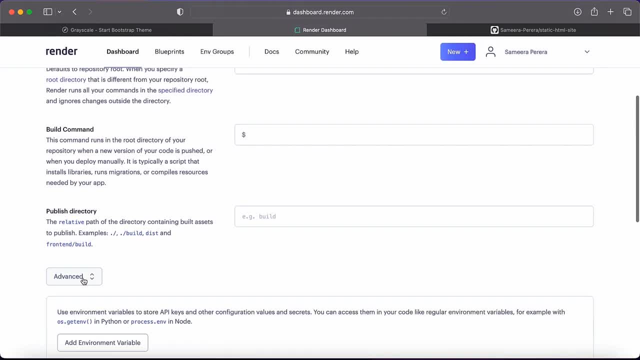 go for different product options here and here i am just making settings with the rooms on my command. the host system is dedicated because basically here is like ake go and the apis. in here you can see village leads and in advanced settings if you have any environment variable or any other configuration, you can. 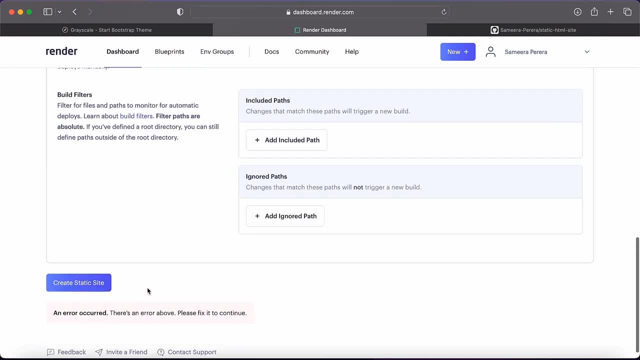 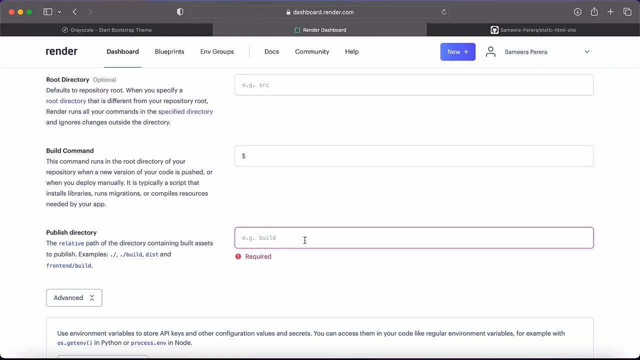 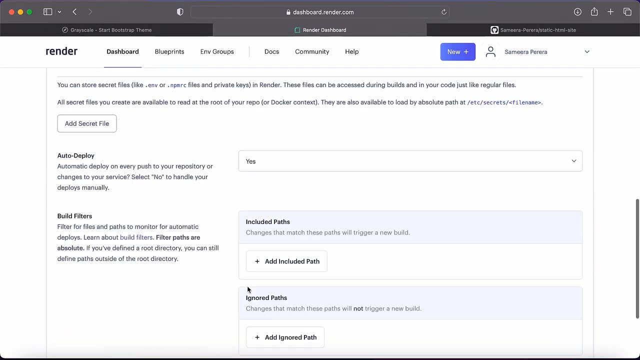 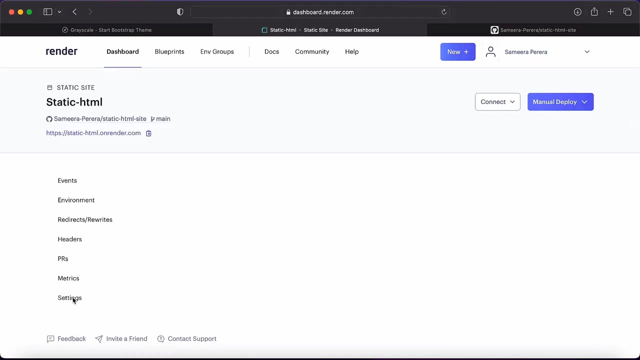 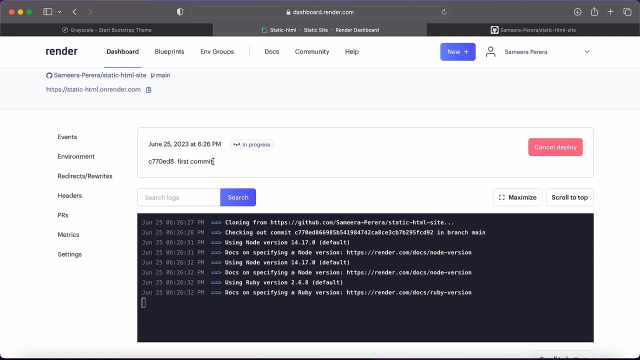 simply set, so i don't have. i have one error. uh, yeah, i have to give public directory. it is just my root directory, so just put the. yeah, this is my root directory. i will put the root directory. that's my public character. just create the application, okay. uh, now it's uh deploying, so it will take around two to five minutes.